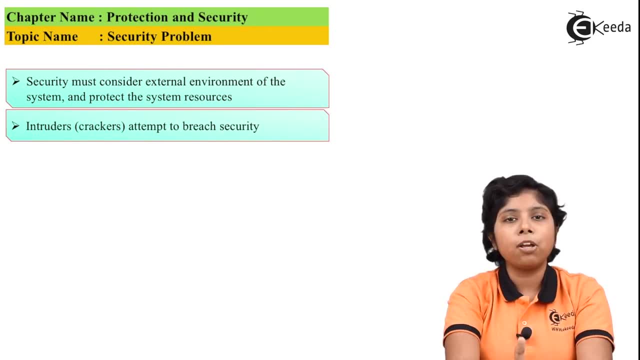 talking about those users who are want to security violet in terms of the breach of confidentiality, availability and breach of construction. Now, when we are talking about another types, that is a threat, we are talking about a potential that is configured to security violation And, finally, the security violation is the attacker. 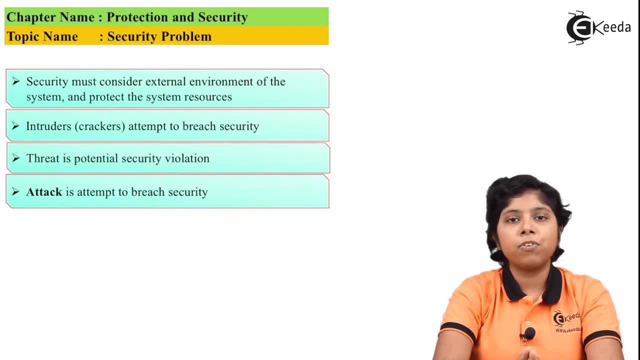 or an attack that is a break to security. So we can see that the attacker want to breach the security via the attack to break the security and this threat is a potential for this vulnerability of the security measures of a system. So we will now discuss the security violations that can happen within a 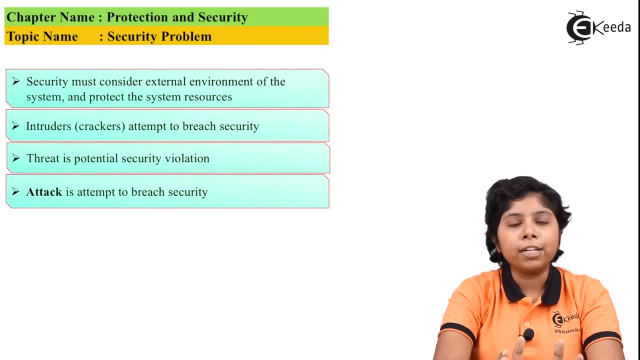 cooperating system. So there is no final and full protection to the operating system that can be measured. But we have to make this prepared So high to the cost that the intruder will be in a jeopardized situation to actually intrude in the system's. 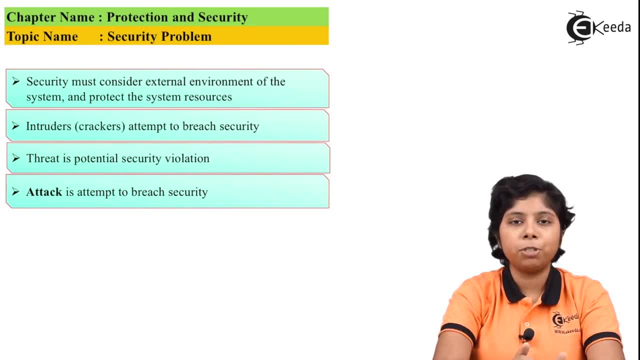 security. So the first type of security information that we will give today is the breach of confidentiality. When we are talking about the breach of confidentiality, that is, the unauthorized read of a particular resource or data, that is say, when a corporation function is mentioned, that only some of its employees 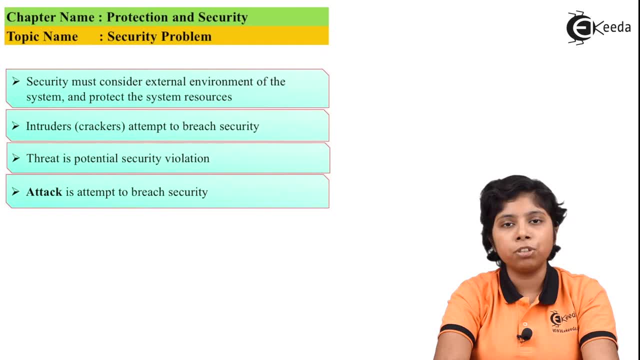 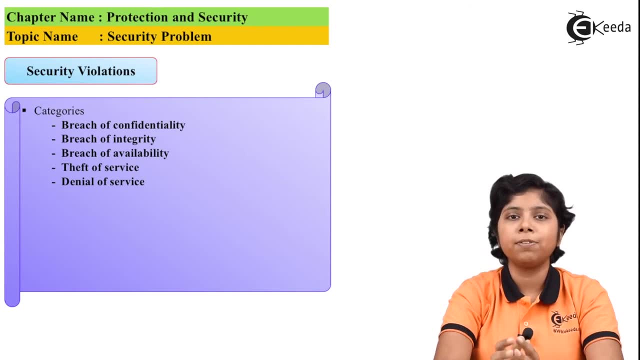 can read the particular data and there lies an intruder which actually read this type of confidential information to breach the violation of that particular cooperative society. You can see that the confidentiality can be breached in the cipher 15, this credit card information or the user's identification information in case of user's authorization. The next type of security violation is the 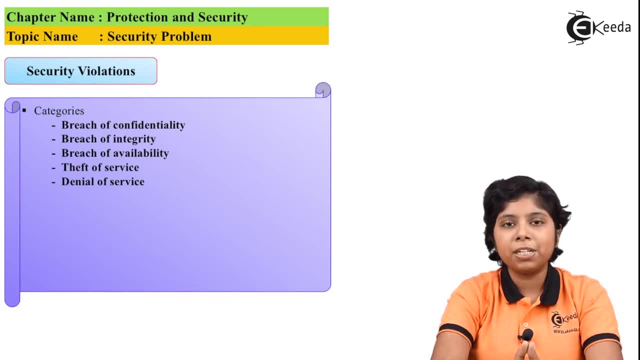 breach of availability. Breach of availability is the unauthorized use that the resource is made to prevent the legitimate use by an authorized access. Say, the attacker wants to green the status or bargain the situation or those privileges that would not be entitled to him normally. So in this case they use the information to 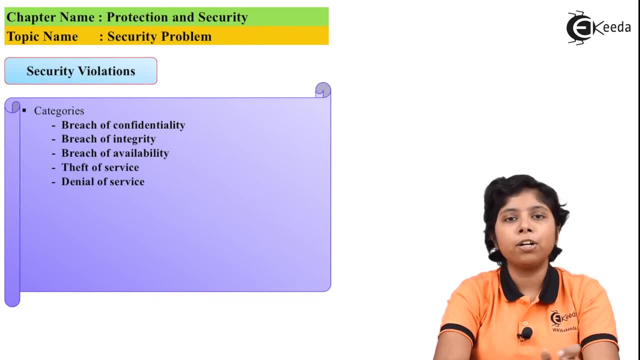 actually get into the status of a particular system to unauthorizedly access that use of the system. The next of the security violation is the breach of modification. The breach of modification constitutes that whenever the user is getting that unauthorized modification of data, say that do install a demon. that is unauthorized in the system. so 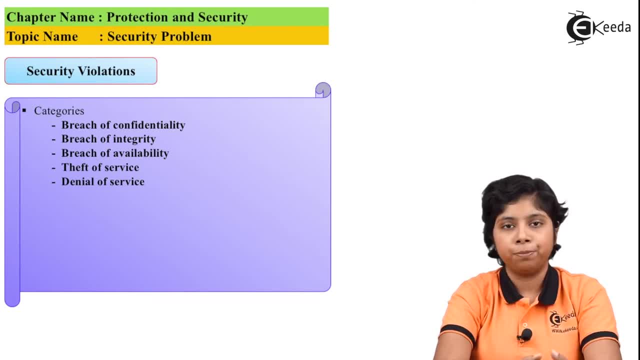 that the system can act as a file server. for that into the. The next type of security violation is the theft of service. So what do you mean of a theft of service? that we are providing the data or the service information to an intruder other than the intended senter? 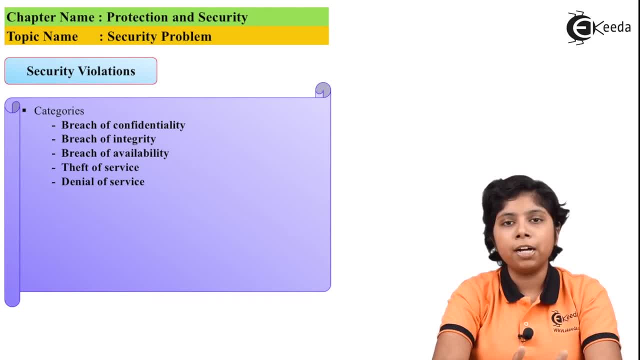 so this intended sender will now receive the data as part of the intruder, because the intruder is gaining or capturing these images of confidentiality information, say for the username and password in a user identity login. and the last type of security violation is the denial of service. denial of service attack is rather an a measure to crack the security that the 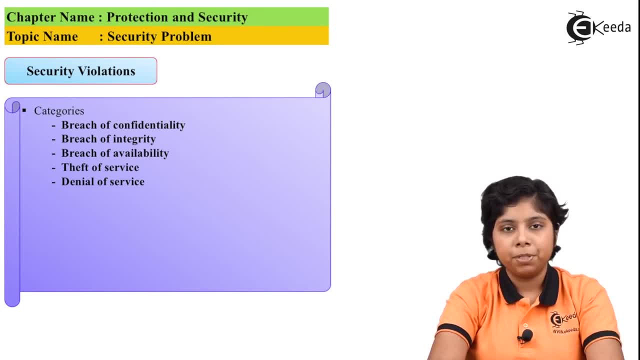 vulnerabilities can happen within our operating system. see when a network is having a corrupted area, so that the communication can be taken and the denial of service is there. if a bug is delayed to fail, spread, and quickly, so the denial of service can measure that counter measure to. 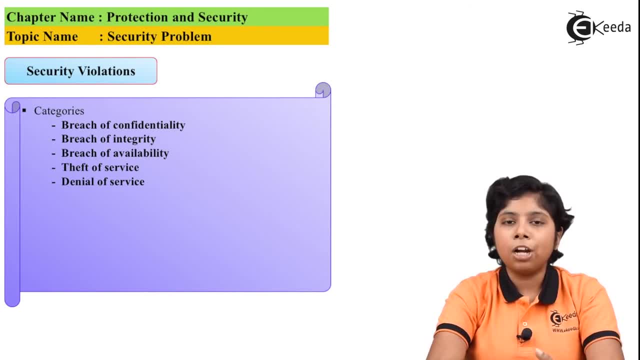 the security violations can be taken. it is allowed to detect such error, but we want to prevent such error by this denial of service attack. now, all the security violations by an intruder or an attacker can be done in many ways. the first process by which the intruder does this is masquerading. what do you mean by masquerading? 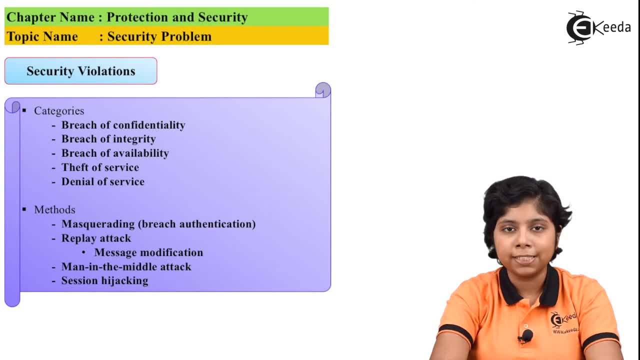 that the intruder becomes, in the communication taking place, that intruder or the participant that is not using that particular mode, say for the sender, which is not an intended sender but actually the intruder. so in this way masquerading can be done by the intruder or the attacker. 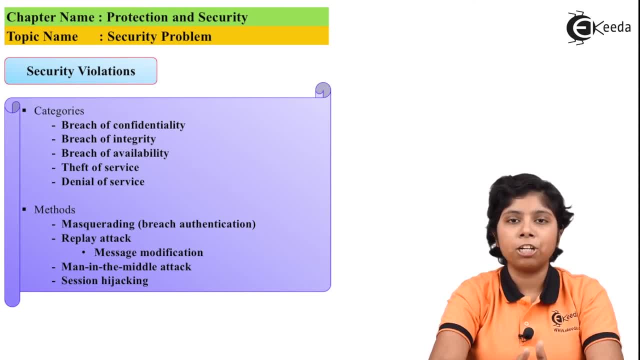 so this masquerading is done by an intruder to actually get this security violations done. so this masquerading is often done in terms of the unauthorized authentication or the correctness of the identification. so now that the intruder want to gain privileges, that was not intendedly. 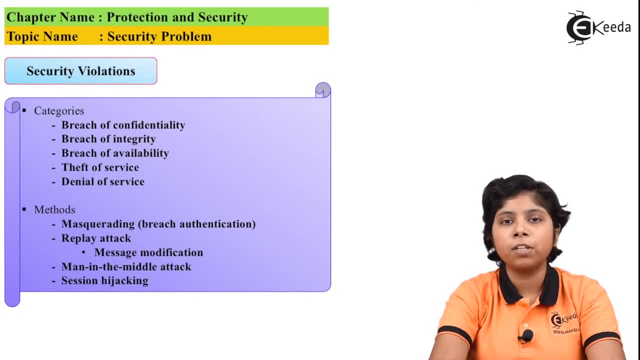 given to her. so it will then theft this implementation of the presentation of this privileges from the user which was intended for that particular use. so the second process by which the user can get this security violations done is the replay attack. by this replay attack, the replay of a particular repeated information is doing by the intruder. 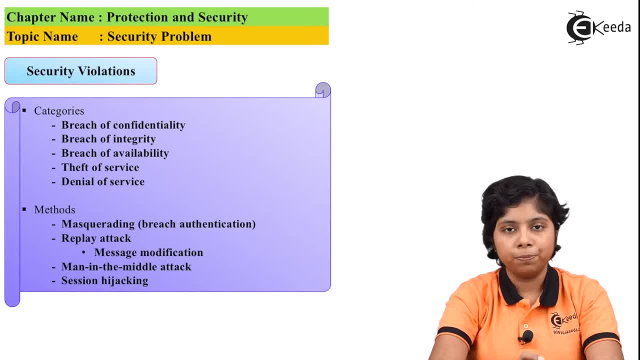 say that it is being replayed that the user authentication which is being given or a legitimate access by the user. so this replay attack is often done with the message modification: say, when we are turning this repetition of requests for money transfer, the user authentication of a legitimate user is replaced by the unauthorized access by an intruder. 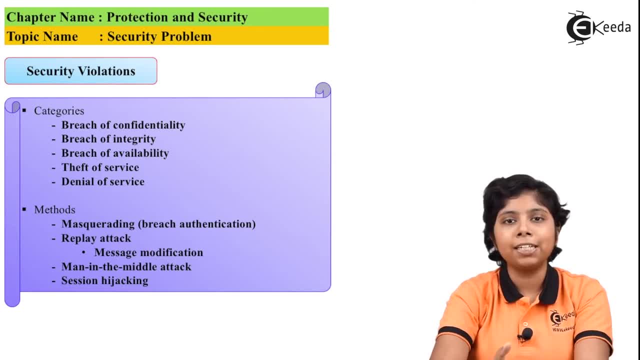 so the intruder gets into the account of the user and then can use this account as the intruder's choice. next type of the introduction done is a man in the middle attack. this man in the middle attack first the intruder gets in the communication that is taking place. 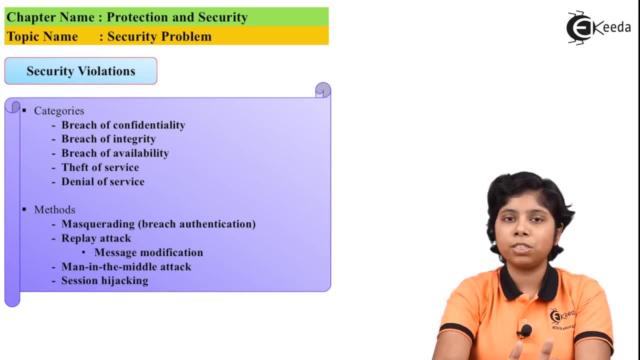 between a sender and a receiver, and then it's access the receiver for the sender and the sender for the receiver. so in this way it's become a man in the middle which is attacking both the sending and it again eruptiously changes the data to send it to the receiver. 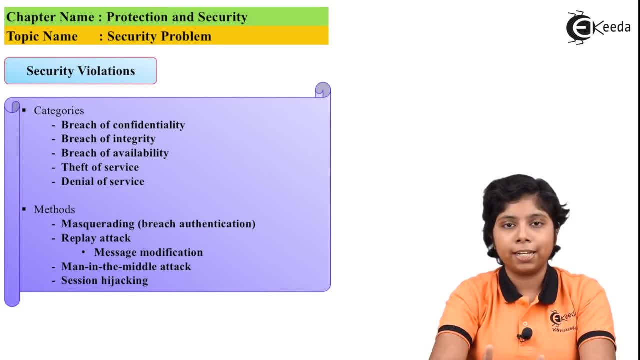 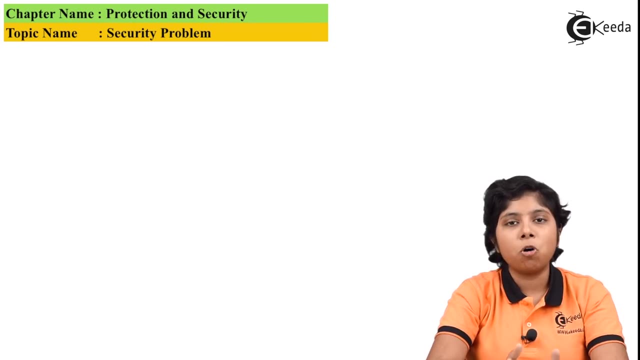 so this often comes with privately, by session hijacking, that a private session was between this private of sender and receiver. now been hijacked by the intruder to get in the man in the middle. now, as we have already told that the operating system or the machine and the human cannot give the protection at this fullest, 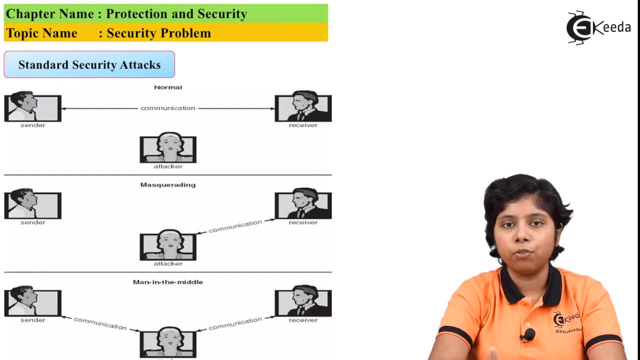 but we should take measure like this security violation or the counter measures, so we can say that we are giving a security breaches at rear rather than it will appear normally. so we can possibly make it a very reducing number so that the security breaches by the intruder cannot get intruded in a particular operating system. 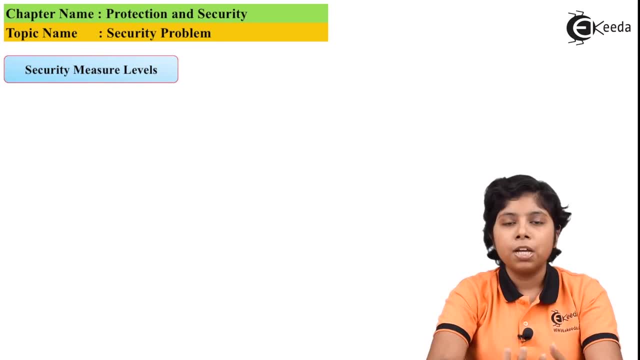 so the measures can be taken in four different levels. the higher level or the high most level is the physical level. in here the sites or sites that is attached within computer system now should be carefully prevented from the unauthorized access, say for the workstations that is a terminal connected to this machine or a machine room could. 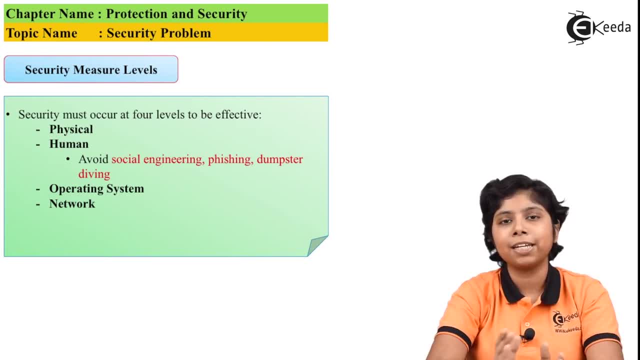 be secured in such a way that no unauthorized access can be done on that particular machine from the physical side. the next higher level of this level of the security countermeasure is a human. by human interaction we can specify that we are preventing an unauthorized access by the user. 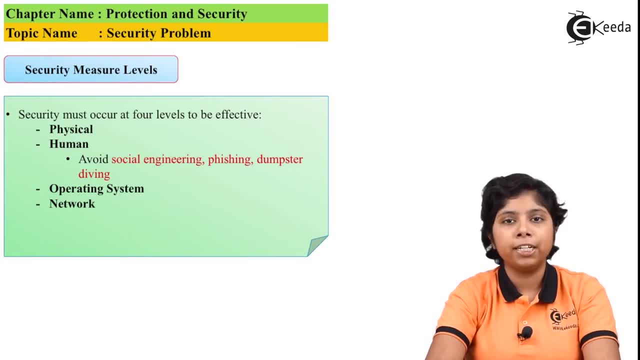 that is, only a intended user can access a particular data in a particular mode. see for the user who is a normal user can given a read mode on that data and a user which is the owner of the data can given a read, write and execute mode on that data. 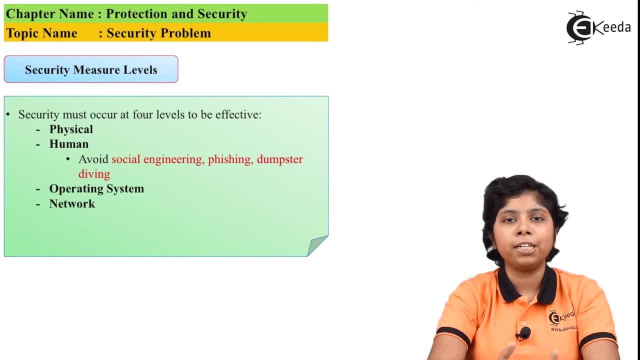 so in this way we can this authorization from getting hacked now, even sometime. the authorized access users will get then the unauthorized access of particular use and the data say: sometimes it can be done accidentally or they are forced to give such confidential information so that the unauthorized access users can gain. 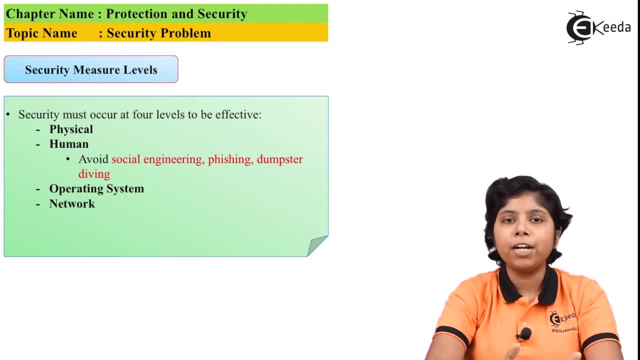 access of that particular privileges. this is often done by social engineering. one type of social engineering is phishing. in phishing it provides why the intruder that is a very legitimate looking web browser or a login program which will force to give the authorized access users to give the input of the 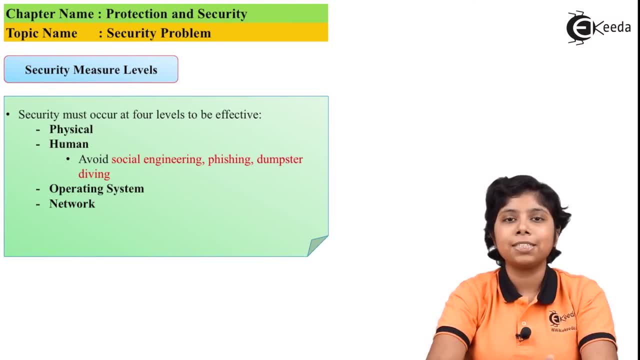 confidential information so that the unauthorized access get taken place. another type of such an engineering is a dumping driven. this dumping driven is performed to collect and gather information, information from a machine that is not properly secured, so that it can gather information from the trash, from the phone, red books or a note containing the passwords. 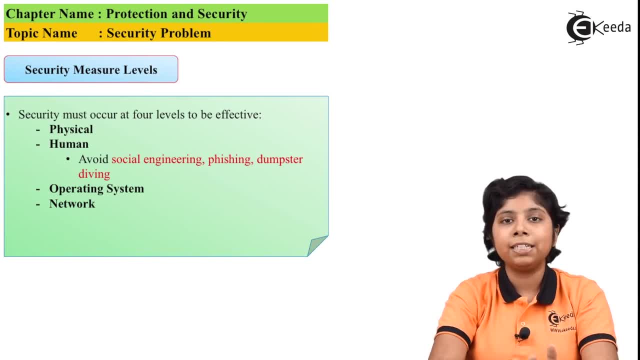 So these are the areas that the operating system cannot handle, and it is done by only human involvement of that particular access. The next level of the countermeasure to security is the operating system measure. The operating system must be secure and independent enough to secure against any types of that. 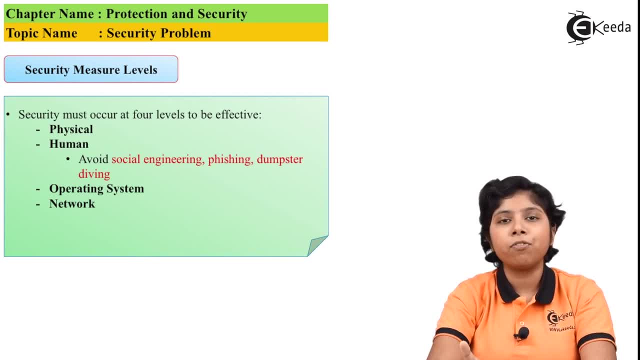 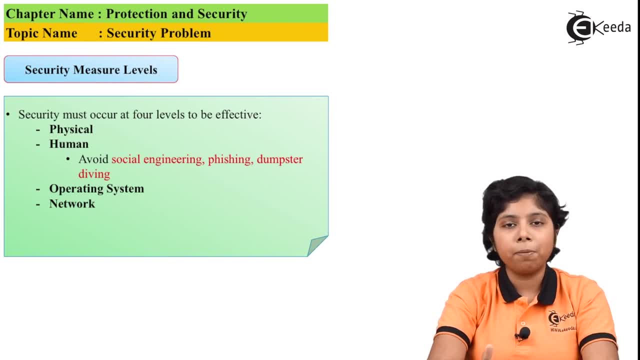 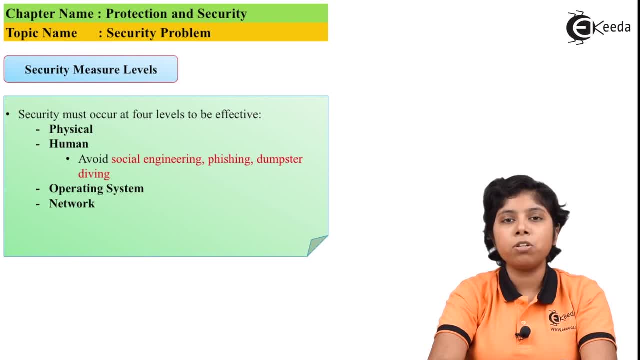 So we need to secure the networks in such a way that they will be used only for the intended purpose. Now, this high, two-level user countermeasures which is to be taken place in security is to be done at the most secure level Because if there is weakness in the higher levels, like the human intervention and the 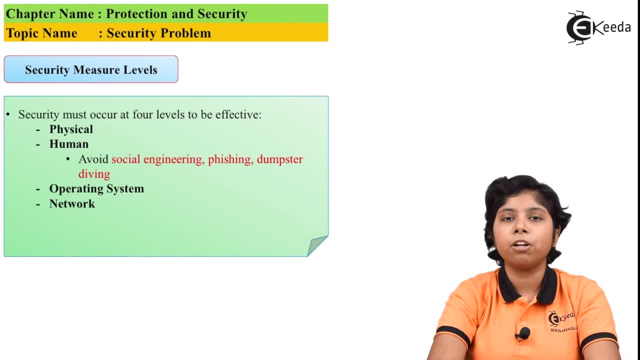 physical measures, then it will affect the low-level security measures at most, like the operating system and network layers. So we need the human intervention and the physical sites or the physical programs in the applications of the operating system to be secured at its most. Furthermore, the system must provide protection to make actual use of the security measures. 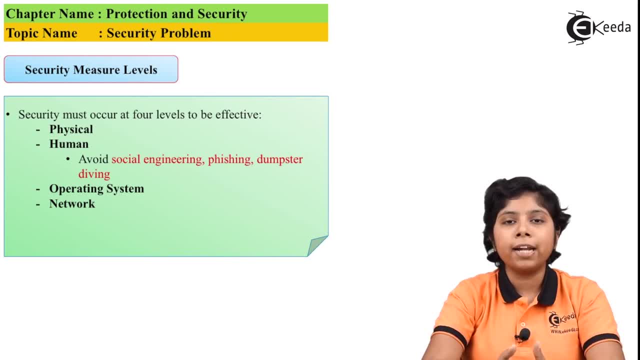 that we have talked about. So, other than using an access authentication of the user, we cannot provide any types of security measures that the user is accessing of the resources, So they need to control their resources, access, their privilege rights and also the access. 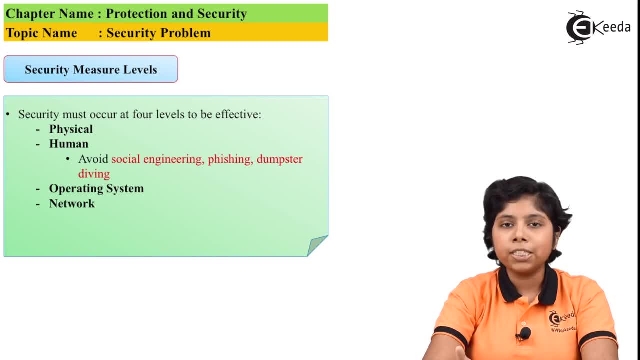 of the memory of that particular data. So in this way, the operating system is used to design in such a way so that the operating system is mostly enough to secure the data that is being used as a resource to the user or the accessor, Such as the memory protection system. 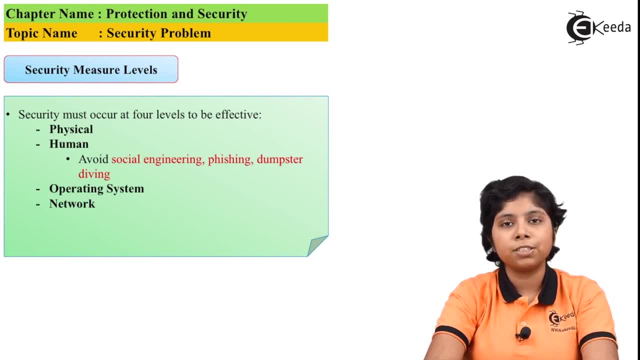 So this is a very important point. The security measures that we need to be given at the operating system level is, at most, necessary for giving any types of security measures, that is, concerning the resources to be stored in that memory system. Now, this giving security measures and taking implementation of it is not straightforward.